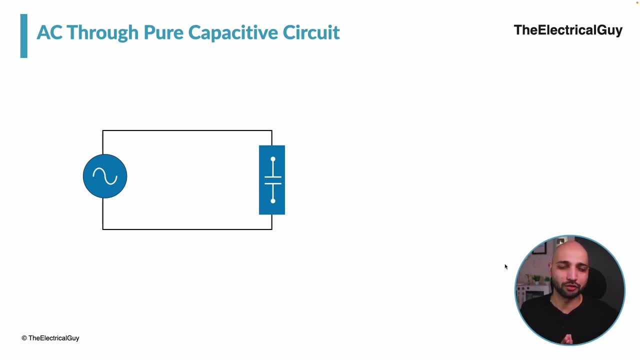 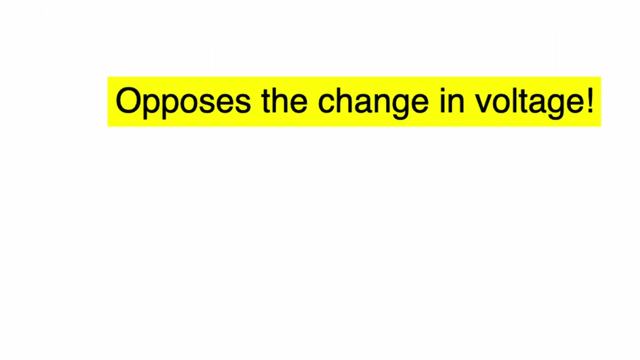 opposite. the change to the flow of electrons. Constant current inductor will allow, but it will not allow any change in the current. that is happening happening. capacitors behave differently than a resistor and inductor. what capacitor does is: capacitor opposes the change in voltage. and how it opposes by supplying or drawing the current. 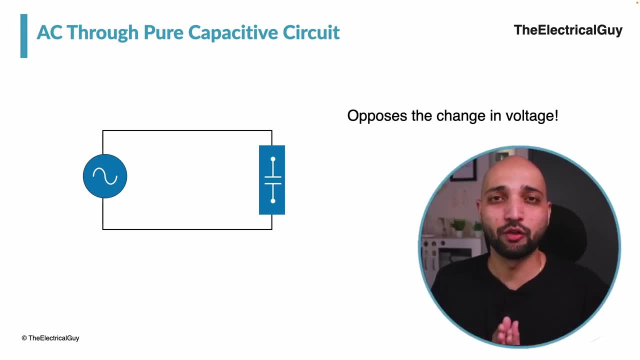 from the circuit. so basically a constant voltage. if you are passing through a capacitor or giving supply of a constant voltage, capacitor is okay, but if the supply is alternating in nature then capacitor will not allow that. it will try to maintain the voltage at a constant level. it. 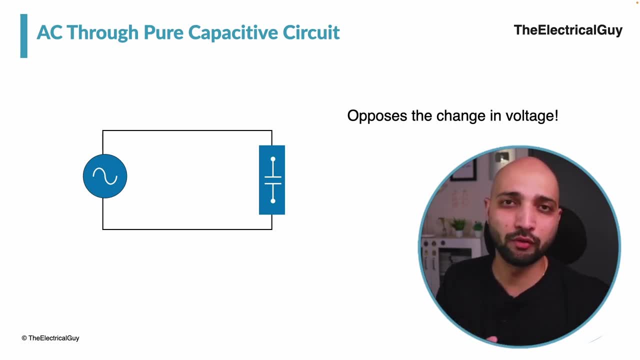 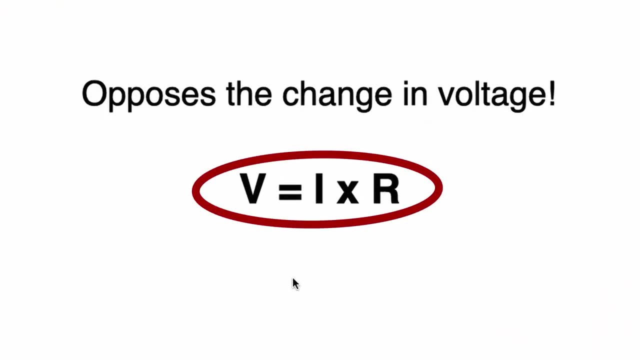 will try to control the voltage and how one can control the voltage. well, again, it takes us back to the ohms law. now what ohms law says is voltage is directly proportional to the current, provided the resistance is constant. if resistance is constant, then it is pretty much sure that 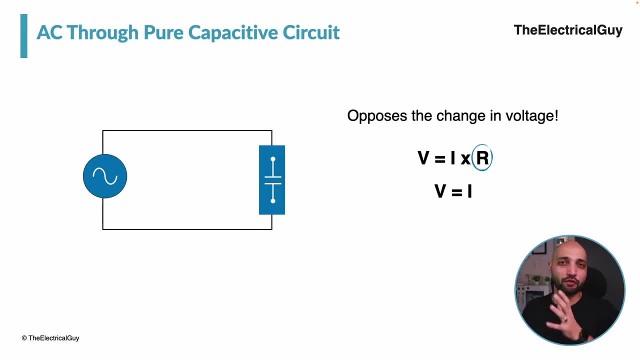 voltage is directly proportional to the current. so if you control the current through the circuit, you can control the voltage. and the same principle is used by capacitor. but before we start, remember we are talking about purely capacitive circuit. now what does a pure capacitor means? it means it has. 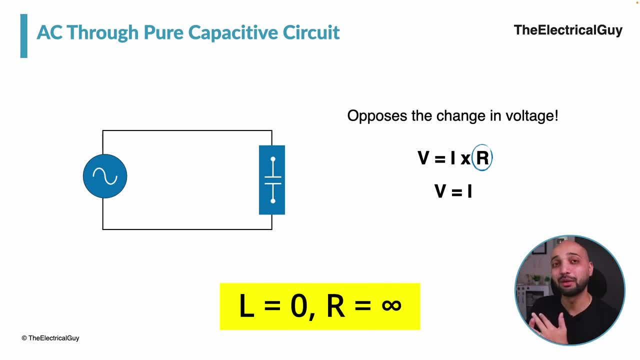 a zero inductance or the zero inductive reactance, but the resistance is infinite. only then we can call a capacitor as pure capacitor and we are discussing everything considering. the capacitor is pure, so we can control the voltage by controlling the current. so whenever we apply an alternating 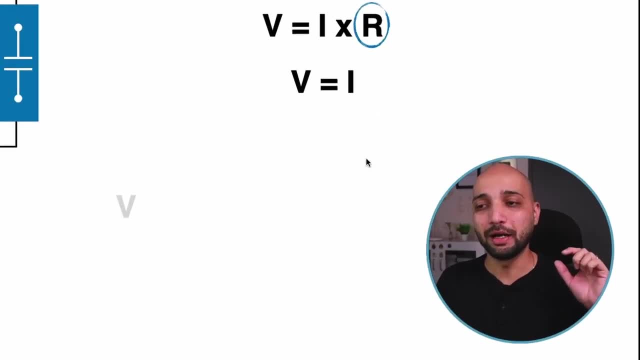 supply to the capacitor and a voltage goes from zero to maximum, what capacitor does is: capacitor drops the current to zero so that the voltage can be controlled or voltage can be brought back to its original position, which was zero, right? so, similarly, when voltage drops from maximum to minimum, what 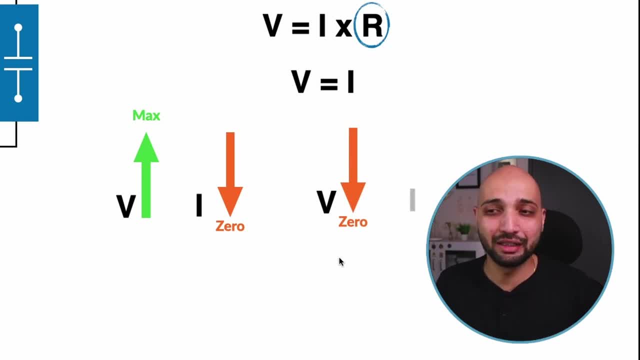 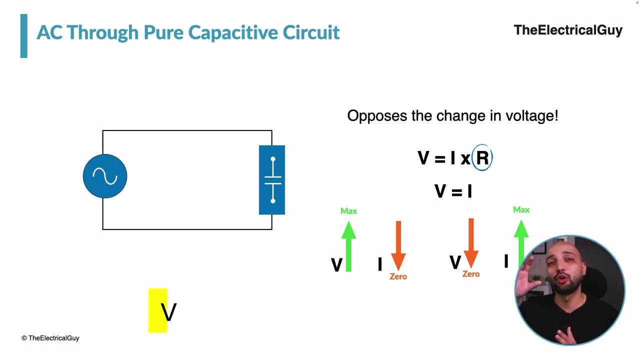 capacitor does is: capacitor pushes the current in the circuit and it takes it to the maximum level so that the capacitor voltage will get back to its previous position, which was the maximum right. clear, understood. and that is the reason why you will see in the capacitive circuit, whenever voltage is maximum, the current is zero. 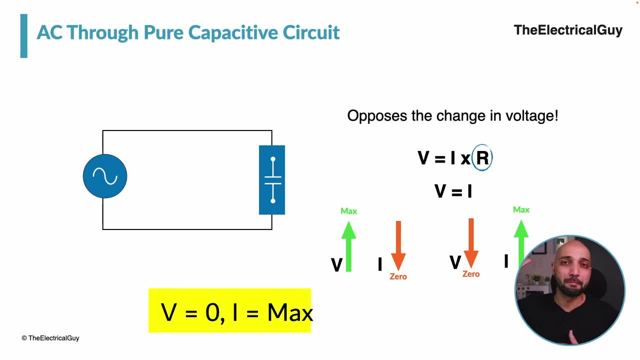 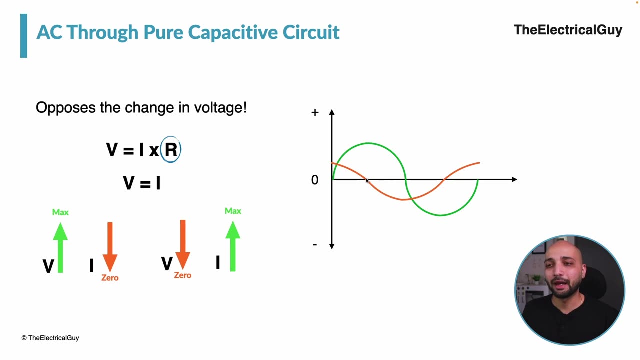 and when voltage is zero the current goes to the maximum level. right understood. now with this we can quickly understand the waveforms of voltage and current in case of capacitive circuit. so here you can see: the green waveform indicates the voltage waveform and the orange waveform indicates the current waveform. so you notice when voltage is maximum. 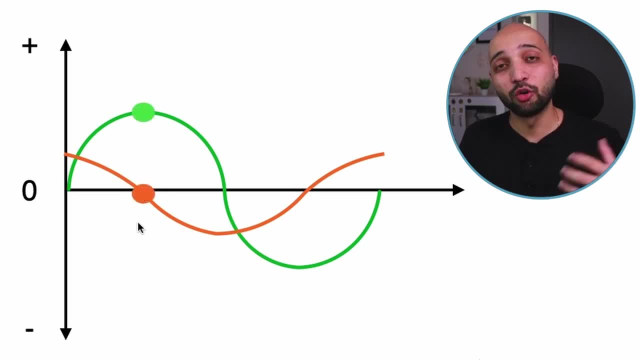 the current is zero. why zero? because capacitor is dropping current so that the voltage can get back to its previous position, which was zero. similarly, in the next position, when voltage goes zero, current becomes maximum. why? because capacitor is pushing more current so that the voltage will again stay or it will go back to its original position, which. 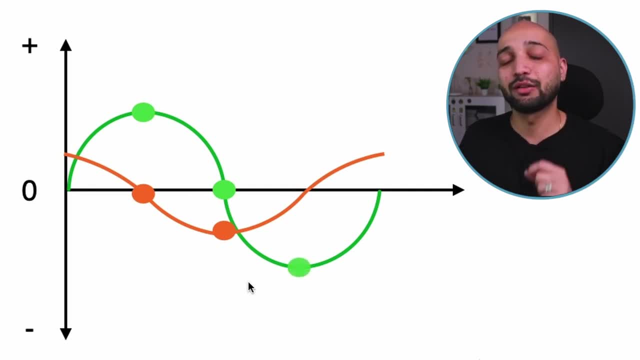 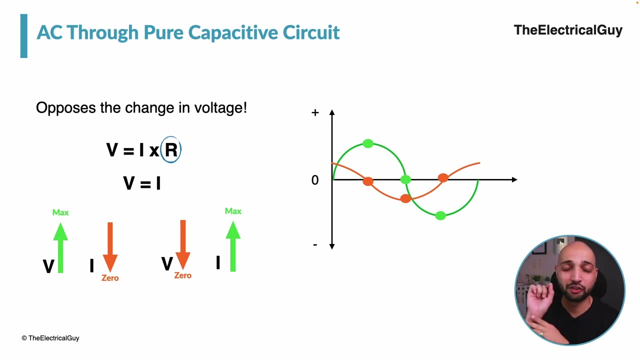 was maximum right. so, similarly, when voltage reaches is negative peak, again the current becomes zero to get back the voltage to its previous position. and hence, if you notice here, when voltage reaches is positive peak, current reaches to its positive peak after 90 degrees right and hence in capacitive circuit. 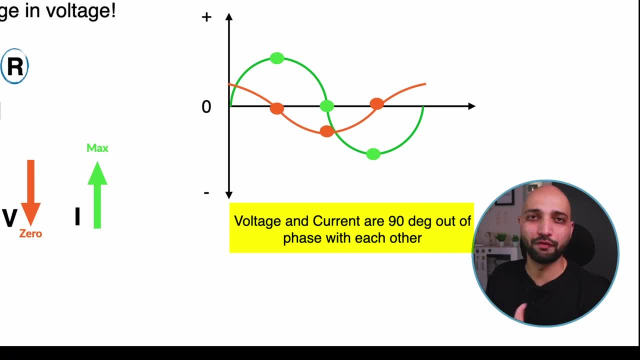 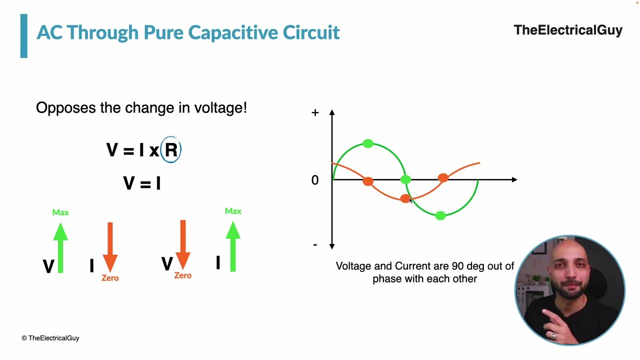 the voltage and current are 90 degree out of phase with each other. so if voltage is reaching to its positive peak at 90 degree, the current will reach at 180 degree. the gap is 90 degree and hence the voltage and current are out of phase by 90 degree. in capacitive circuit we can also say current has a head start. 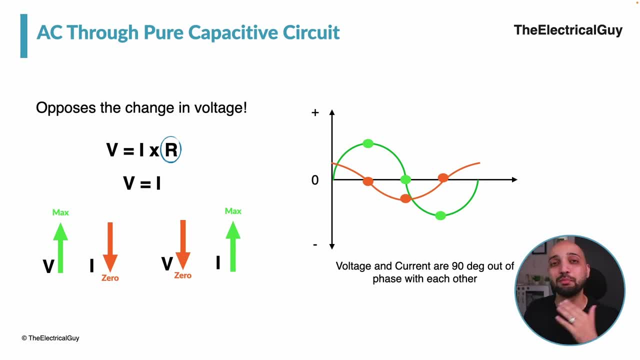 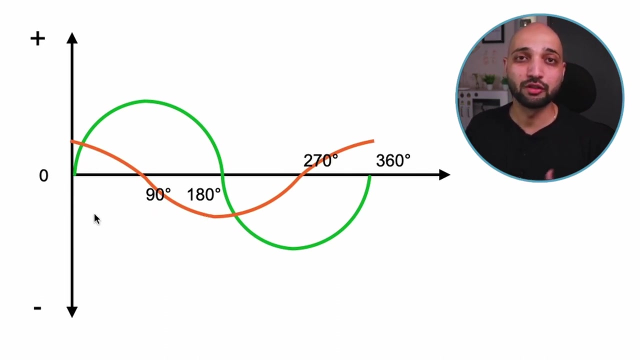 in case of capacitive circuit and voltage lags behind the current by 90 degree clear. this is about how voltage and current behaves in capacitive circuit. now the interesting part: we are going to discuss about the power in case of capacitive circuit. so if you notice the first portion- 0 to 90 degree- both voltage and current are positive. so, of course, 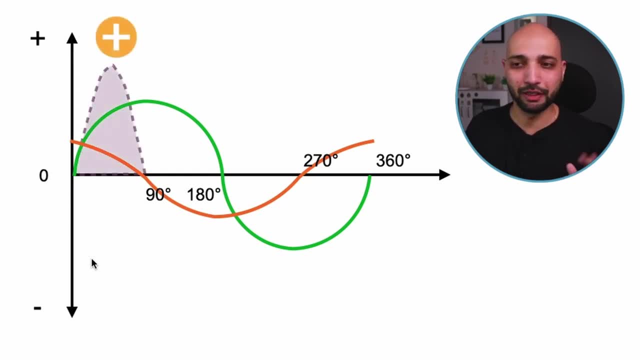 the resultant power will be positive power. that is fine, but when we talk about 90 degree to 180 degree, voltage is positive but the current is negative and hence the resultant power is a negative power, because positive multiplied by negative will give us a negative result and hence 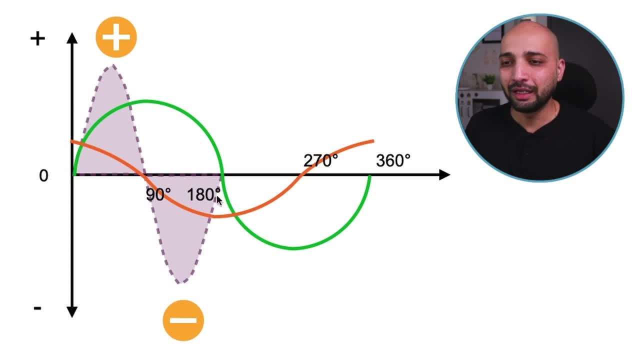 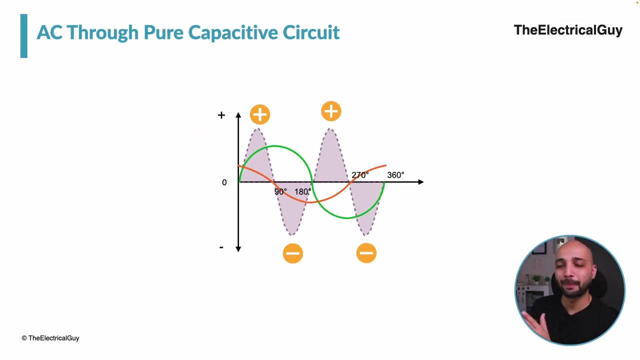 the power is also negative. power in 180 degree to 270 degree, both voltage and current are negative and hence the instantaneous power at this particular portion will be positive. clear in the next phase, 270 degree to 360 degree, the current is positive but voltage is negative and as a result the output power will also be negative. now again, if you 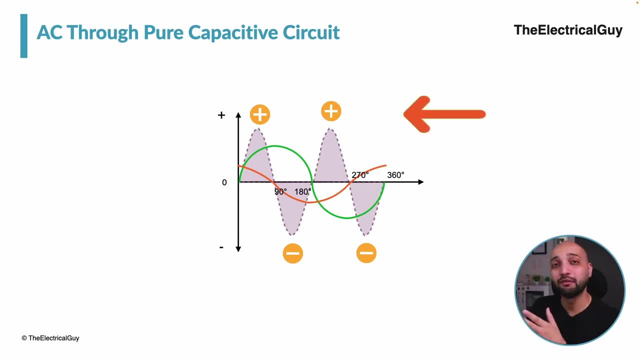 notice: we have two equal positive peaks and we have two equal negative peaks. so these two equal and two- two positive and two negative peaks will cancel out each other and that means capacitor do not consume any actual power. right, positive powers and negative power are cancelling out each other. 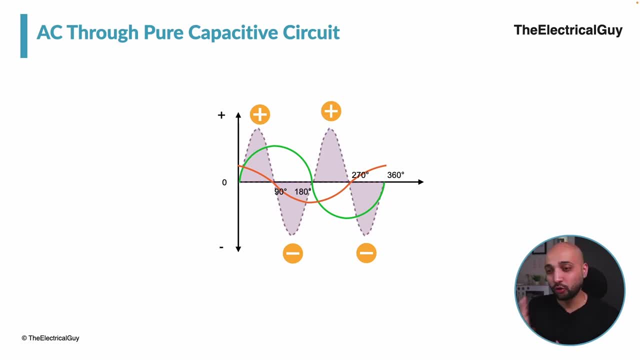 the resultant power remains negative, zero. now first let's understand what is this negative power? negative power means capacitor is delivering power back in the circuit. the positive power indicates capacitor is consuming the power from the circuit and negative power indicates it is supplying power back in the circuit. 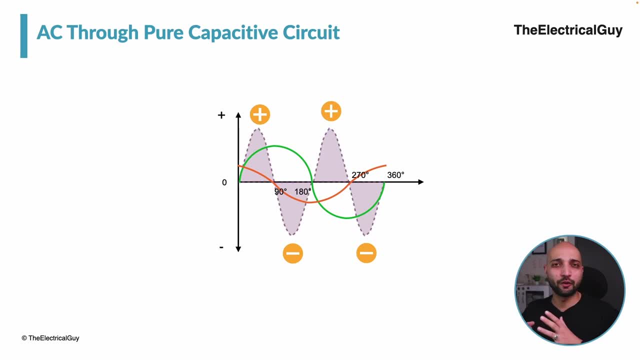 and such type of power, when it goes to the positive, peak, negative peak, positive, negative. such type of power is what we call as a reactive power or imaginary power, the same situation which we saw in the previous video wherein we discussed about the inductive circuit. it is exactly the same situation, but there is one big difference here. 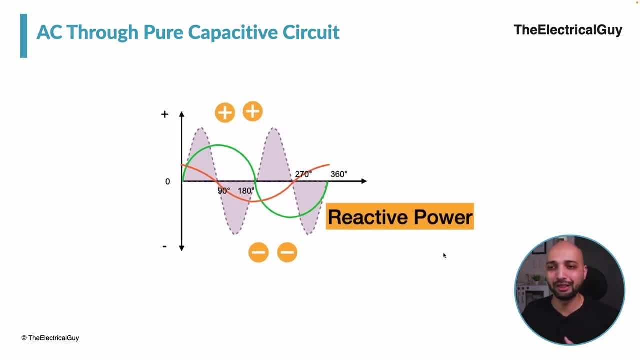 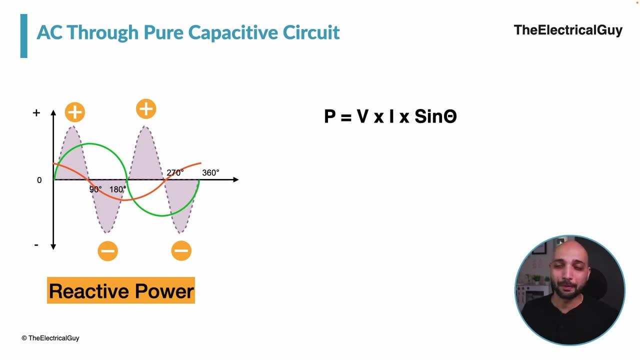 now, if you calculate uh, the power, mathematically, let us, let us do that here. so it is. we saw p is equals to voltage times, current times sine theta. now the theta, that is angle between voltage and current, here is negative 90 degree y in the uh. 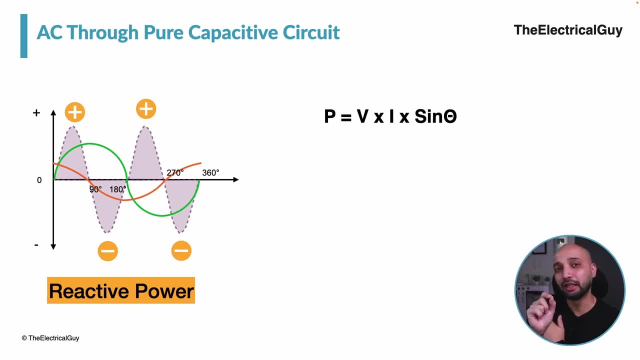 previous inductive video we saw that in inductive circuit voltage leads the current right and hence it is positive 90 degree. but in this case voltage lags current by 90 degree and that is the reason why we have to consider negative 90.. always remember that generally students get confused. 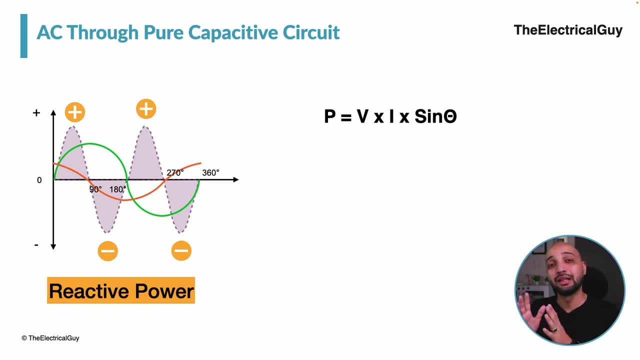 between positive and negative 90.. capacitive circuit: it is negative 90 degrees. so if you put that voltage times, current times, sine 90 degree, the resultant is negative one, the negative one, the value of sine is sin 90 is negative one. so the resultant power will be negative voltage times. 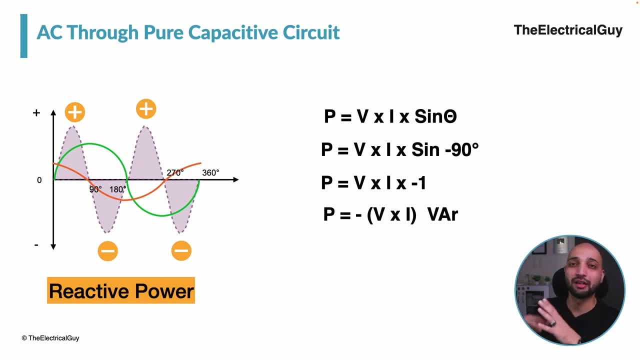 current volt ampere reactive. again, it is a reactive power. hence the unit is volt ampere reactive or kvar, kilovolt ampere reactive. again, since it is a negative power, we cannot indicate it using letter p. we have to use letter q. p is later used for active power only and q is used 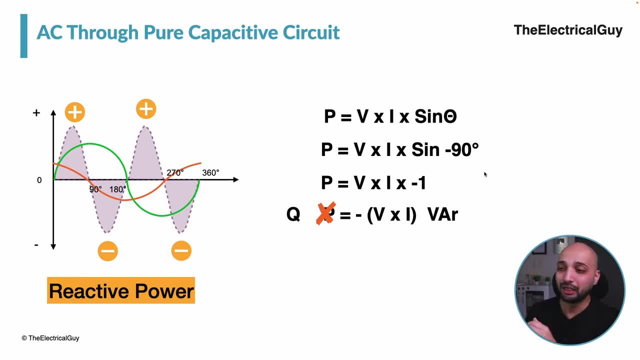 to indicate reactive power, right, but if you notice here, the power, the reactive power here is actually a negative power. and what does this negative power indicate? it means the capacitive circuit is supplying power back to the circuit and not actually consuming it from the circuit. that is the significance of indicating the power as negative. and if you are more interested in in: 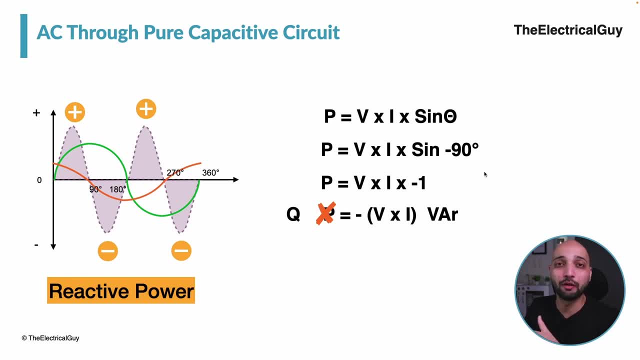 knowing about, uh, reactive power. what does this reactive power mean? where does this reactive power go in the circuit? i have a dedicated videos on that. i'll put link for those videos down in the description. you can go and check that out. and because of this property of capacitive circuit, 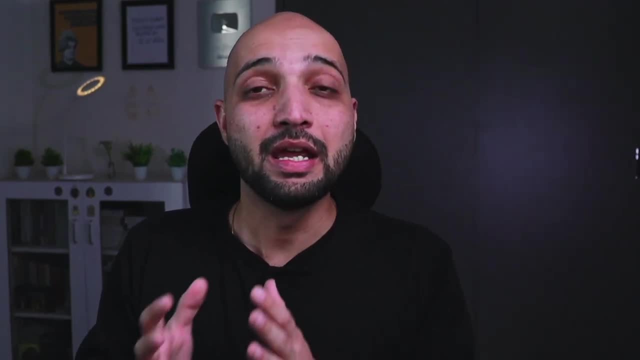 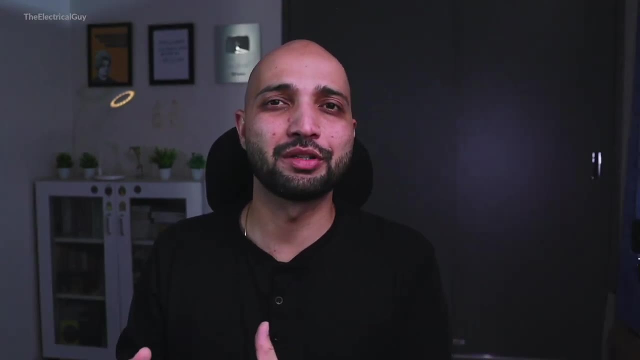 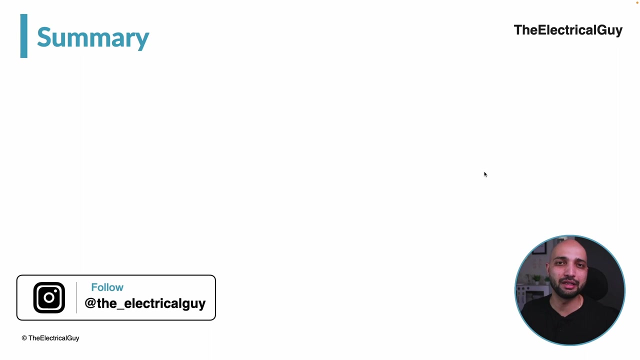 wherein they can supply reactive power to the circuit. capacitor banks are specifically installed in the power system to improve the power quality. the purpose of capacitor banks is to supply the necessary reactive power to the circuit and to supply the necessary reactive power to the circuit. now let us quickly summarize the video, what we have discussed so far. capacitor opposes the change. 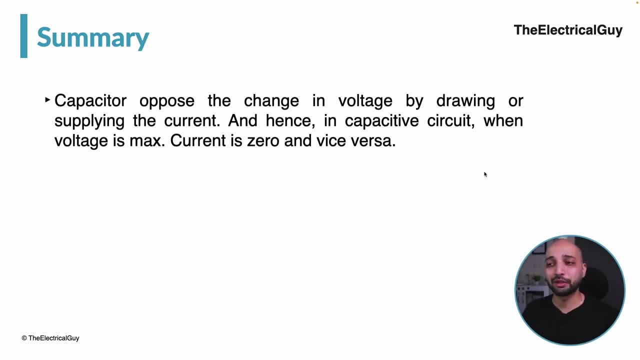 in voltage by drawing or supplying the current and hence in capacitive circuit. when voltage is maximum, current is zero and vice versa. in capacitive circuit, voltage and current are out of phase by 90 degree. purely capacitive circuit do not consume real power. capacitive circuit supplies power back. 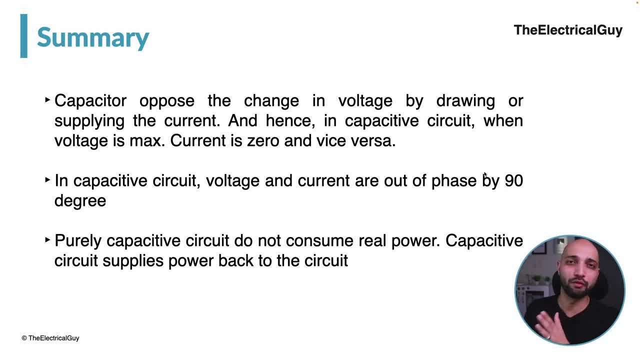 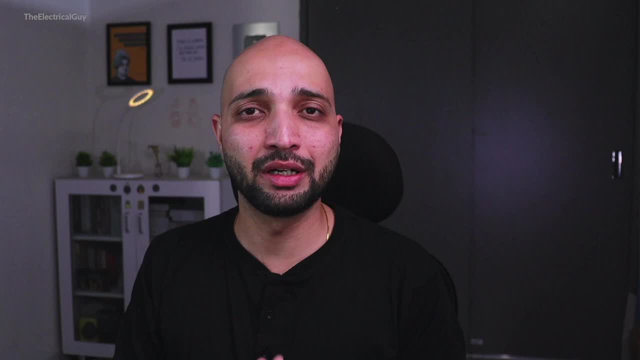 to the circuit, which is again exactly opposite than what we have seen in the inductive circuit. inductive circuit consumes the reactive power and capacitive circuit is supplying power back in the circuit. so i hope you understood something useful today, if the video helped you in understanding the concept. 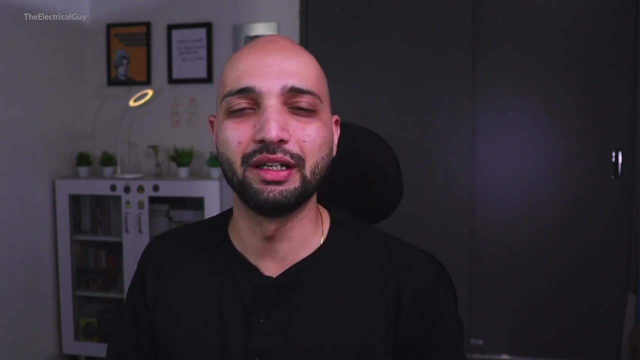 please do like the video and do share it with the electrical engineers. you know that really helps the channel to grow further and i really, really appreciate that. and if you don't want to miss any of the updates of such videos, please do like the video and share the video with your friends and